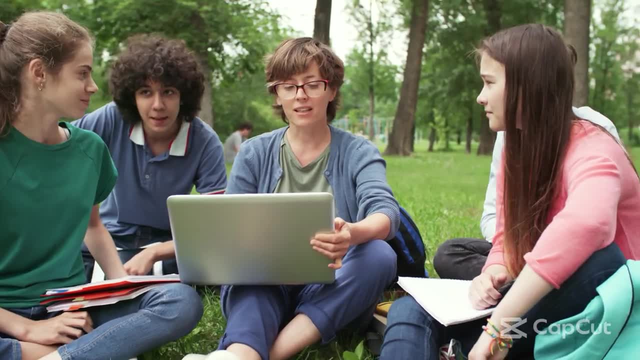 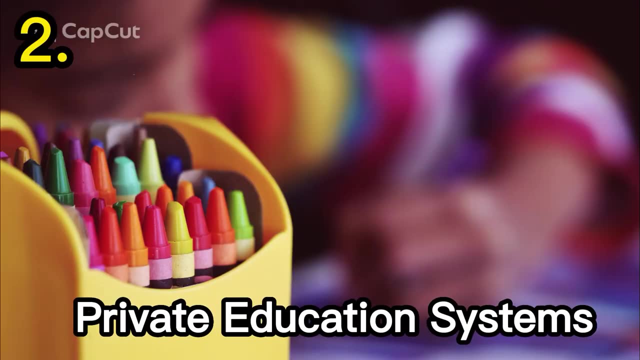 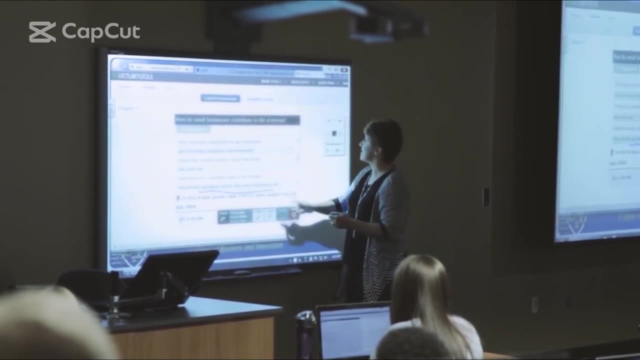 and are usually free for students to attend. In some countries, students may have to pay for certain items such as books or uniforms. 2. Private education systems: these are funded and run by private organizations or individuals, and students usually have to pay tuition fees to 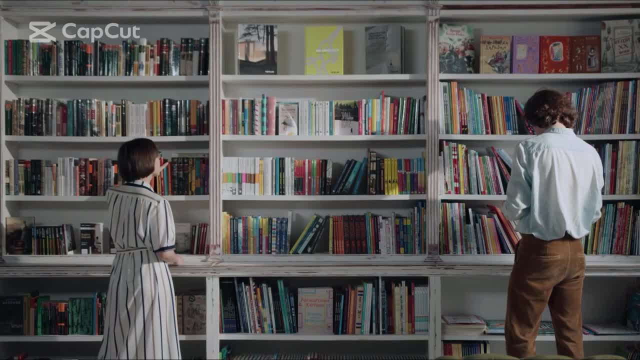 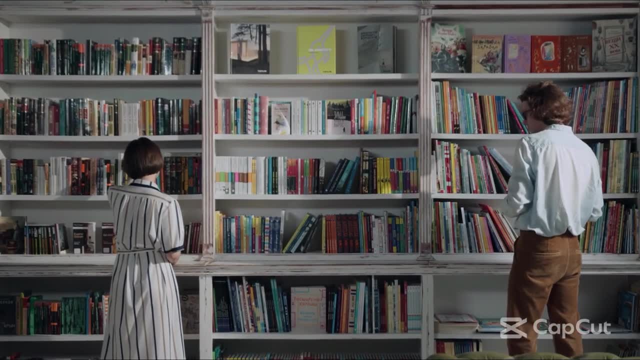 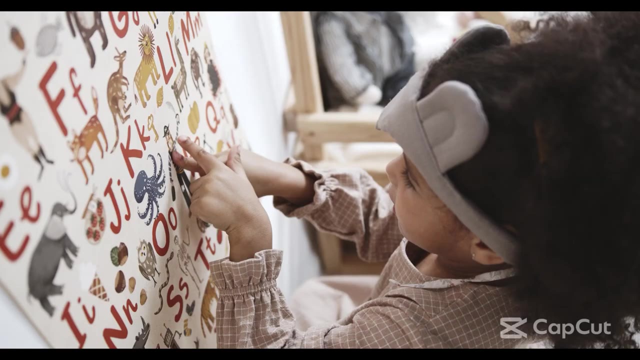 attend. 3. Charter schools: these are publicly funded schools that are run by private organizations or individuals. They are usually given more freedom to experiment with teaching methods and curriculum in exchange for meeting certain performance goals. 4. Homeschooling: this is 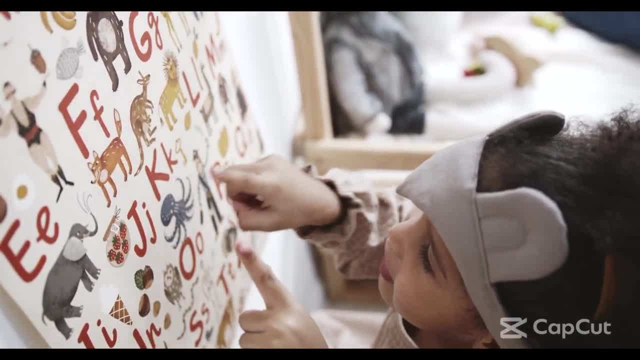 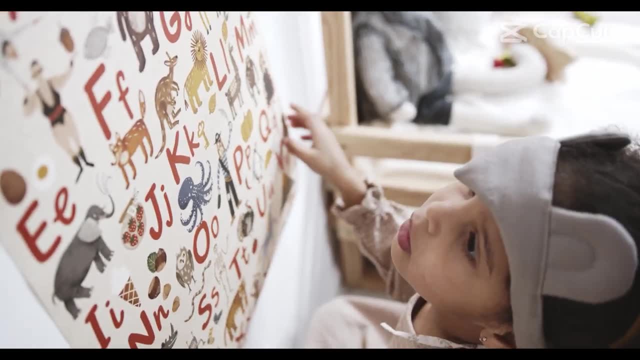 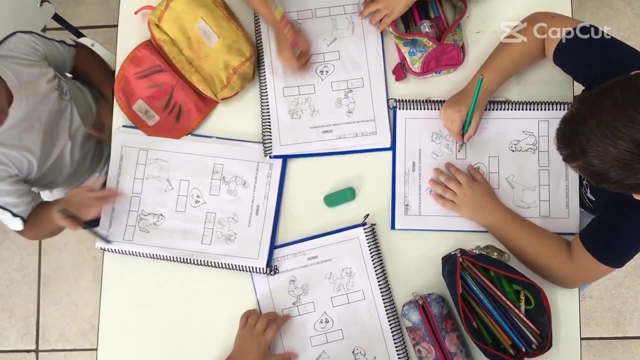 when children are educated at home rather than at a traditional school. Parents or tutors are responsible for providing the education, and the curriculum and teaching methods can vary widely. 5. International schools: these are private schools that follow a specific curriculum, such as the International Baccalaureate or the British Curriculum. 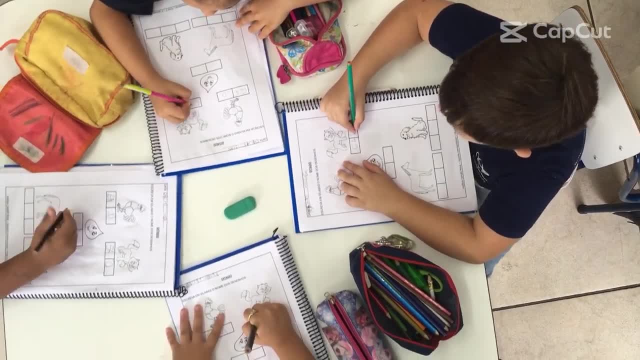 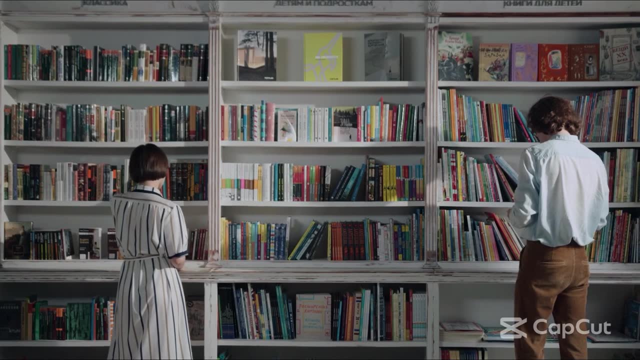 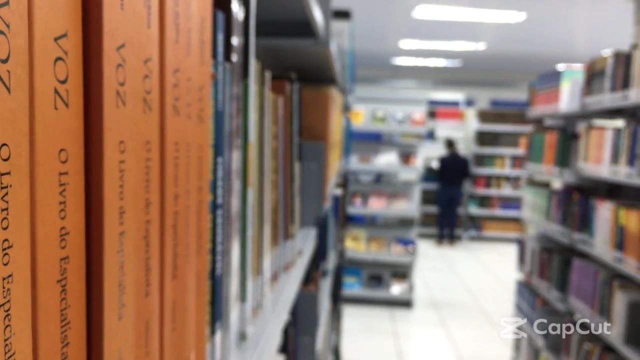 They are often attended by the children of expats or diplomats. 6. Compulsory education: many countries have laws requiring children to attend schools that are not funded by the government. These are often attended by the children of up to a certain age, usually between 5 and 18 years old. 7. Primary education: this is the first. 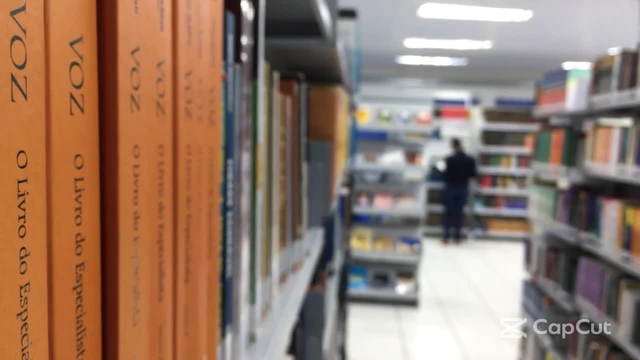 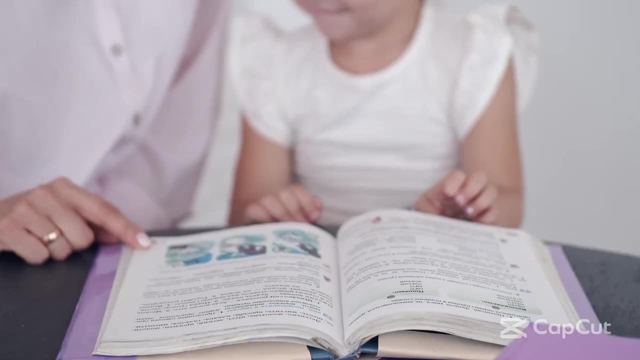 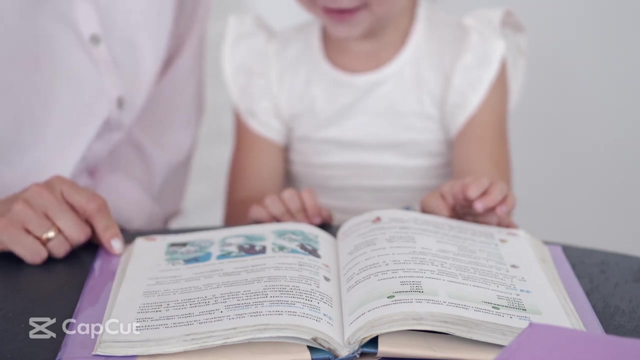 stage of formal education and usually covers ages 5 to 12.. It is followed by secondary education. 8. Higher education: this refers to education beyond secondary school and can include vocational training, associate's degrees, bachelor's degrees, master's degrees and doctoral degrees. 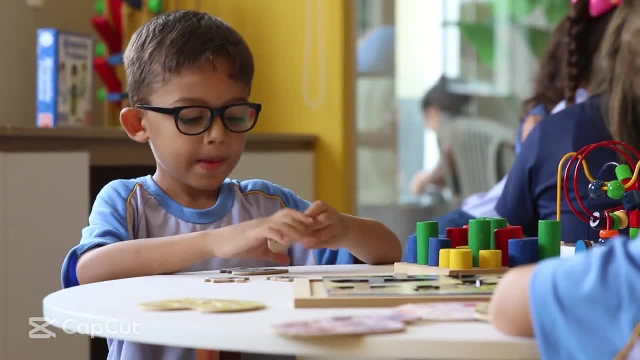 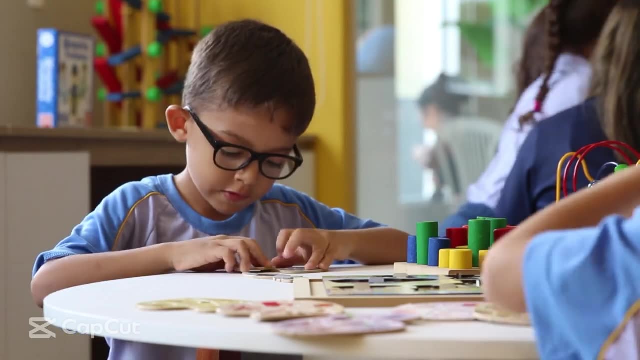 9. Curriculum: this refers to education beyond secondary school and can include vocational training. This refers to the subjects that are taught in a school or educational program. Curriculum can vary widely between different countries and educational systems. 10. Grading systems: different countries and educational systems use different methods to 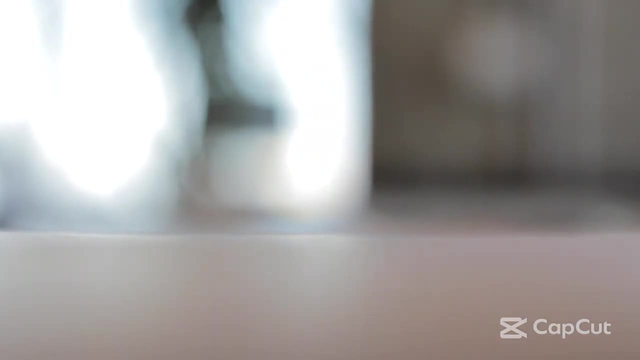 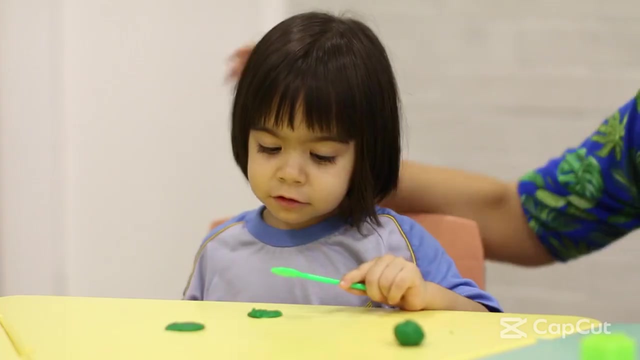 evaluate students' performance. These can include letter grades, percentage grades or pass-slash-fail systems. 11. Standardized tests: these are tests that are given to students to assess their knowledge and skills in a particular subject. 11. Standardized tests: these are tests that are given to students to assess their knowledge and skills in a particular subject. 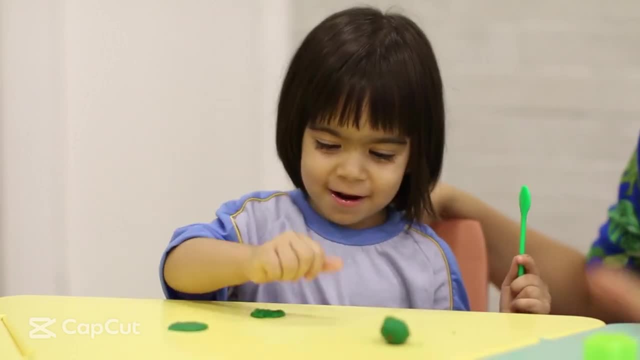 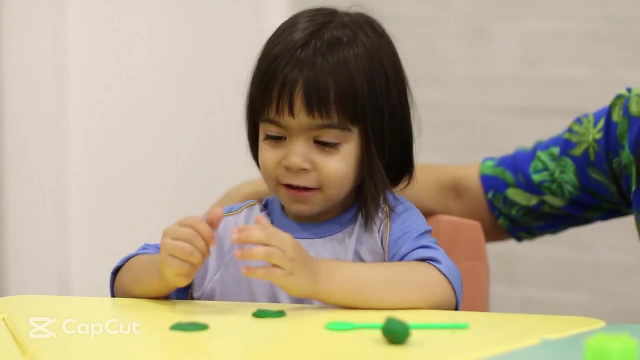 Standardized tests are used in many countries to measure student progress and to compare the performance of different schools. I hope this additional information is helpful.